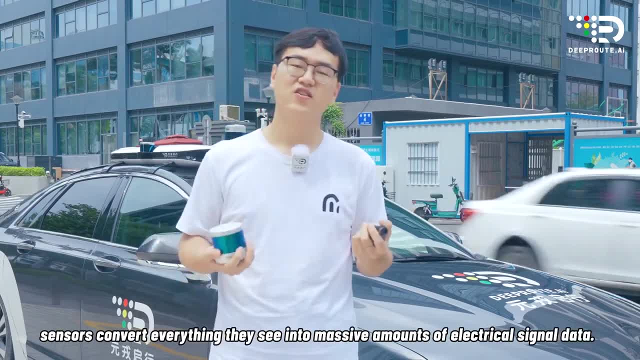 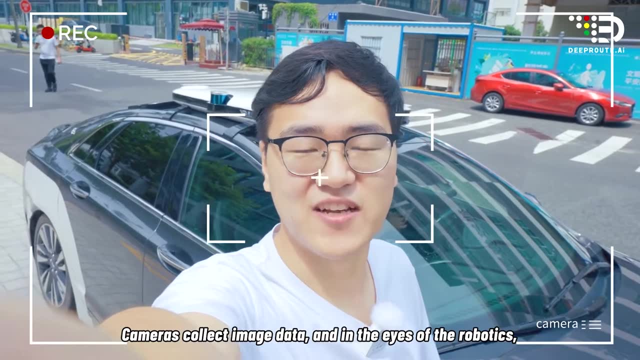 traffic regulations to pass the driver's license test. Sensors convert everything they see into massive amounts of electrical signal data. Cameras collect image data and, in the eyes of the report, they can see what the car is doing and what the car is doing, So the car can detect. 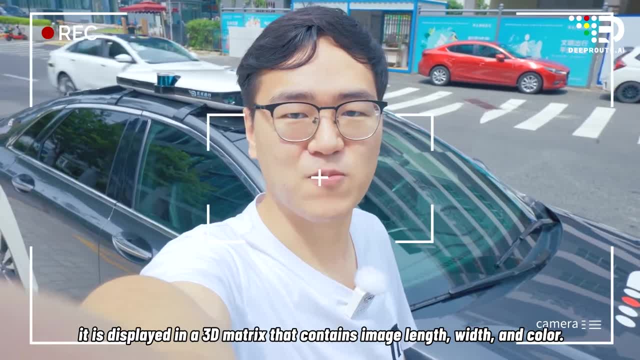 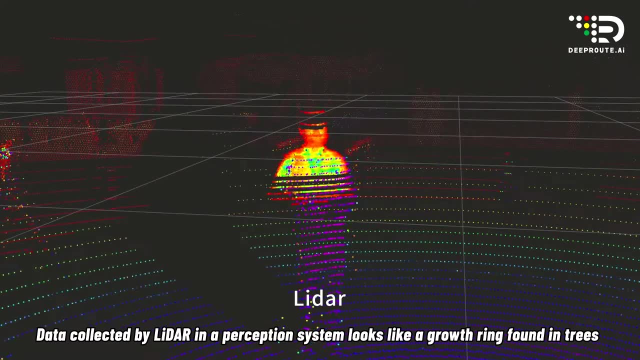 obstacles and roads and understand traffic regulations Only with a clear and accurate understanding of the robotics. it is displayed in a 3D metric that contains image, length, width and color Data collected by LADAR in a perception system. looks like a ghost-ruined fountain trees. 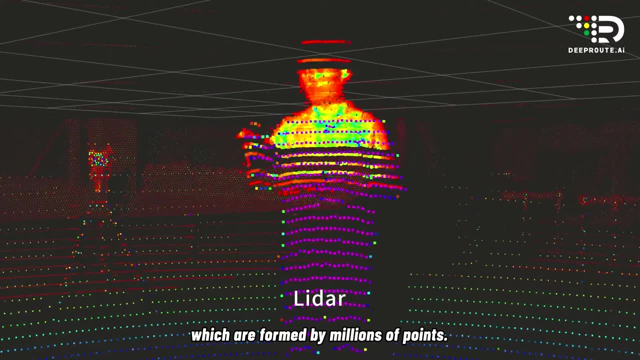 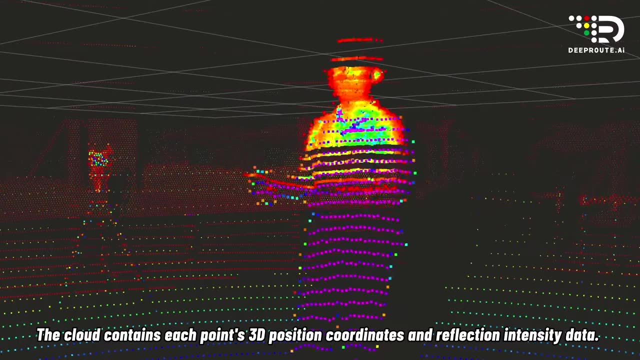 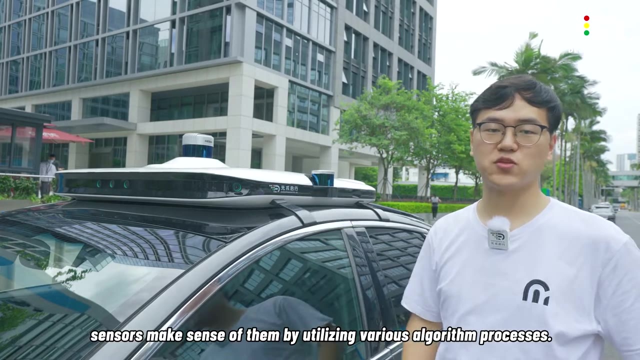 and are called laser point clouds, which are formed by millions of points. The cloud contains each point's 3D perception coordinates and reflection intensity data Based on all the data seen by the eyes. sensors make sense of them by utilizing various algorithmic processes In R&D. we categorize them into two parts based on their parts. 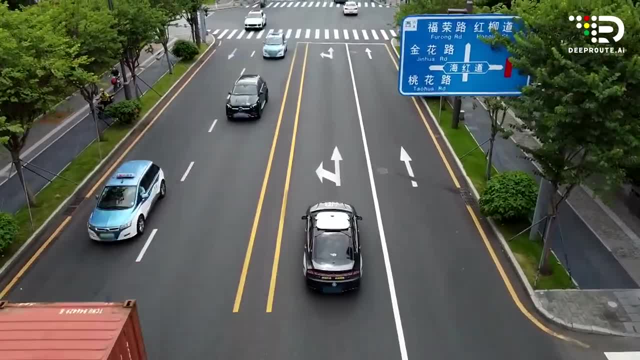 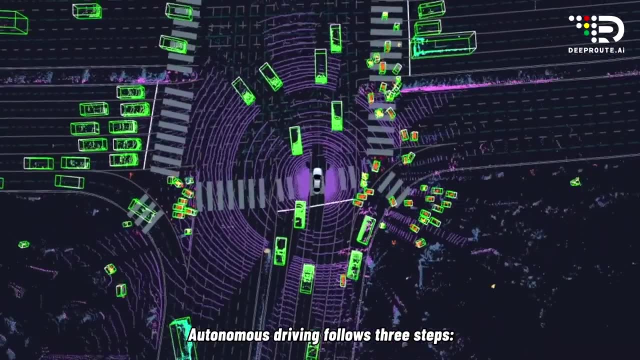 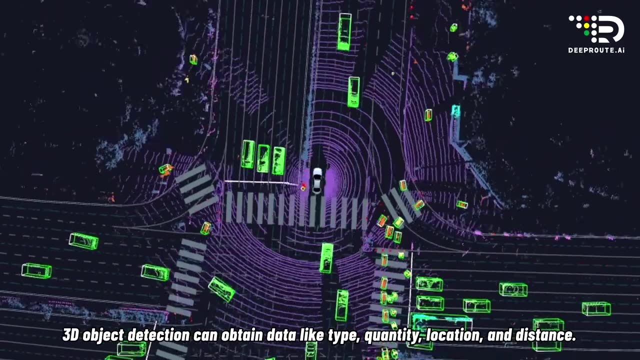 obstacle perception and environment perception. 4. Obstacle perception is the detection of all the obstacles on the road. Autonomous driving follows three steps: detect, track and predict. 3D object detection can obtain data like type, quantity, location and distance. Then, with tracking, the velocity, 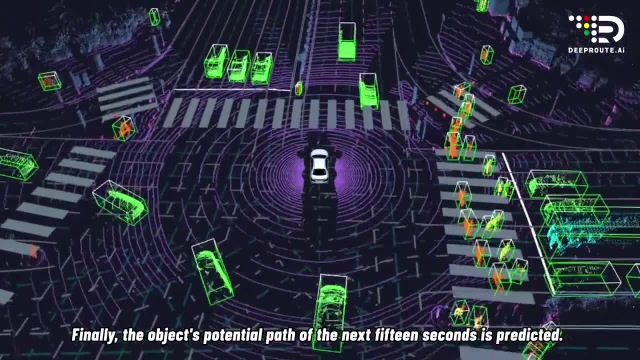 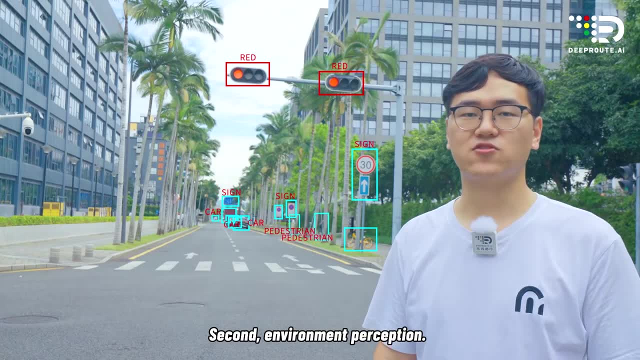 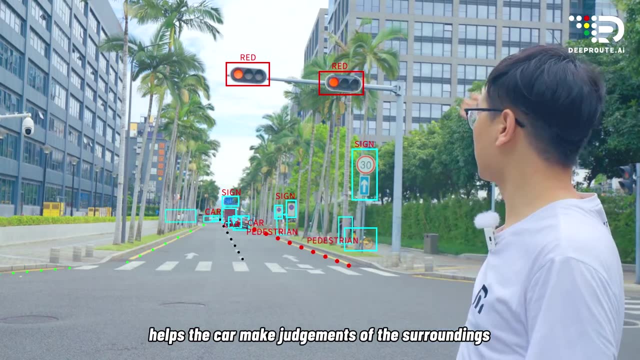 and speed are calculated for more accurate detection. Finally, the object's potential path over the next 15 seconds is predicted. 2. Environment perception. Perceiving and understanding road lengths, traffic signs and road signals helps the car make judgments of the surroundings. 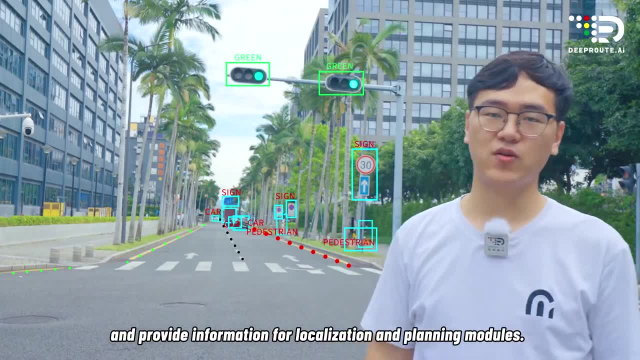 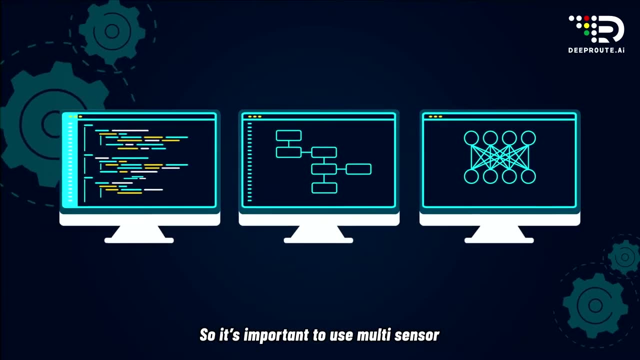 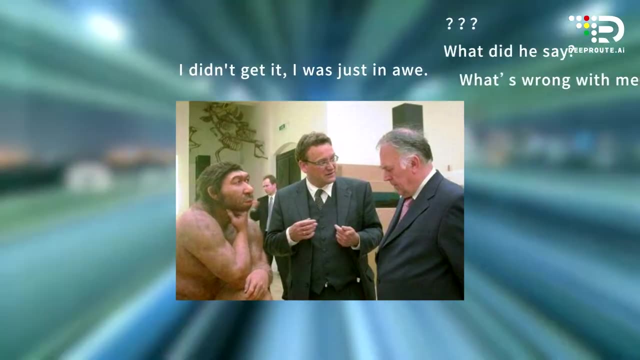 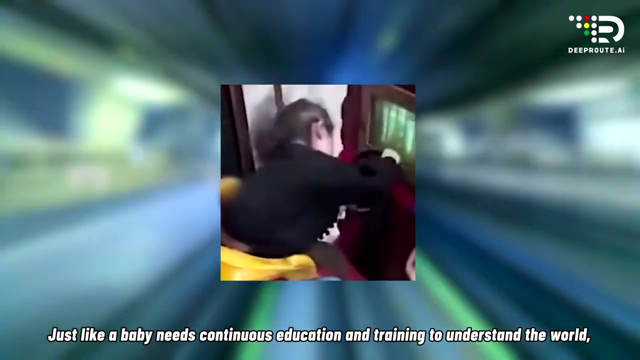 and provide information for localization and planning modules. The same task may have different effects with different data and algorithms, so it is important to use somatic sensor and algorithm fission to achieve more precise perception results. Just like a baby needs continuous education and training to understand the world, 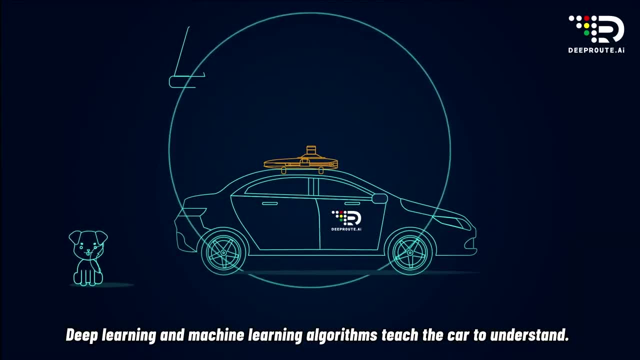 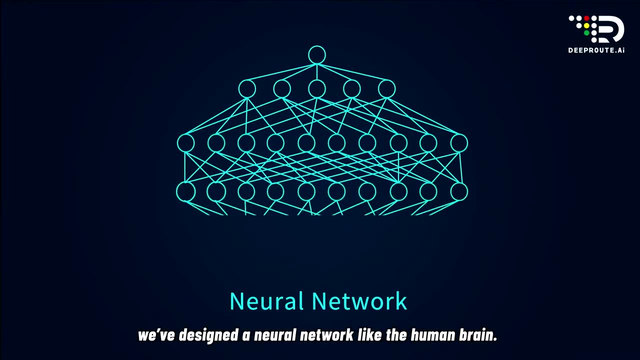 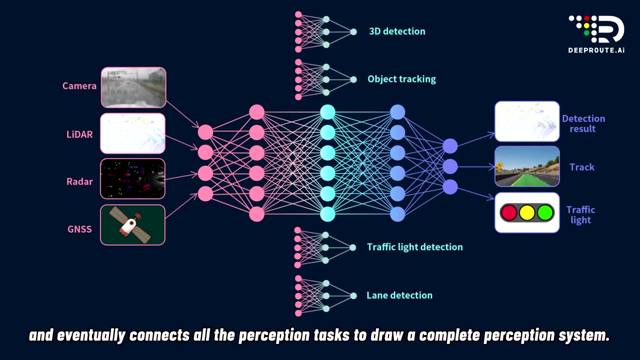 so does the self-driving car. Deep learning and machine learning algorithms teach the car to understand. Based on different perception tasks, we have designed a neural network. like the human brain, It receives training through massive group data, which which deepens its understanding of the environment and eventually connects all the perception tasks.